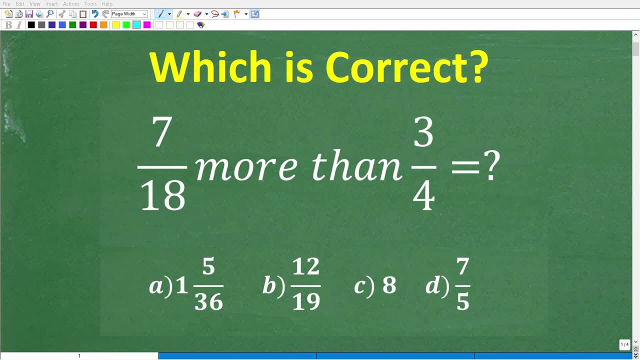 Okay, so let's see if you can correctly interpret what this basic math problem is saying And, more importantly, let's see if you can get the right answer without the aid of a calculator. All right, so here is the question: We want 7 18ths, more than 3 4ths. 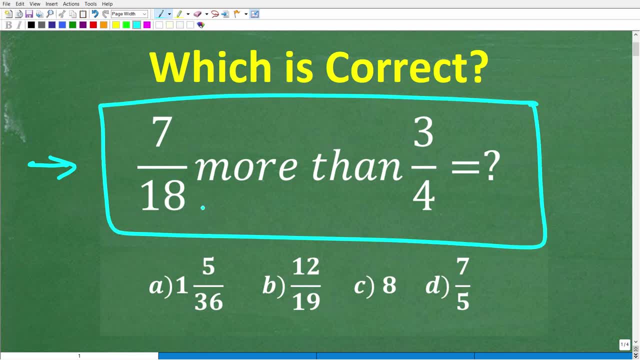 All right. so we have this phrase right here: 7, 18ths, more than 3, 4ths is how much? Well, we have a multiple-choice question here and let's take a look at our answers. So the first choice, A, is a mixed number fraction, so that's 1, 5 over 36.. 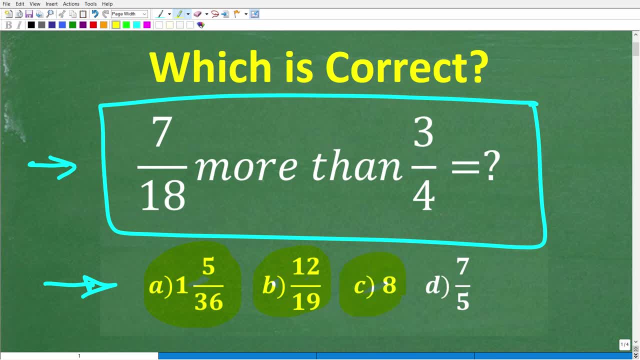 B is 12, 19ths, C is 8, and D is 7 over 5.. All right, so one more time, no calculator, But if you can figure this out, go ahead and put your answer into the comments section. 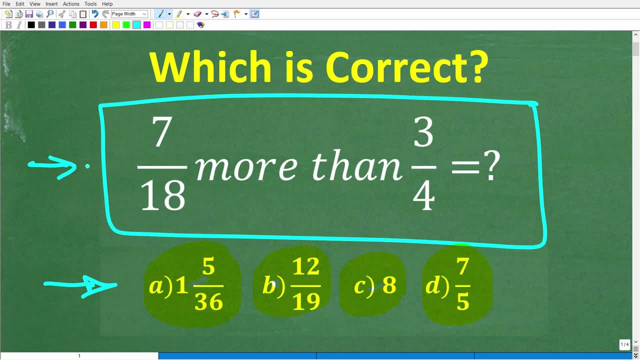 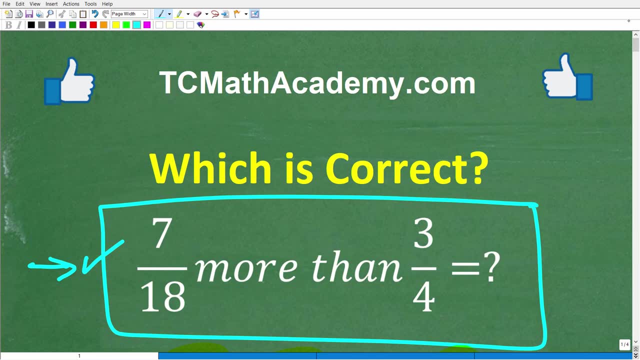 I'll show you the correct answer in just one second. Then, of course, I'll walk through exactly how to solve this problem step by step. But before we get started, let me quickly introduce myself. My name is John and I have been teaching middle and high school math for decades. 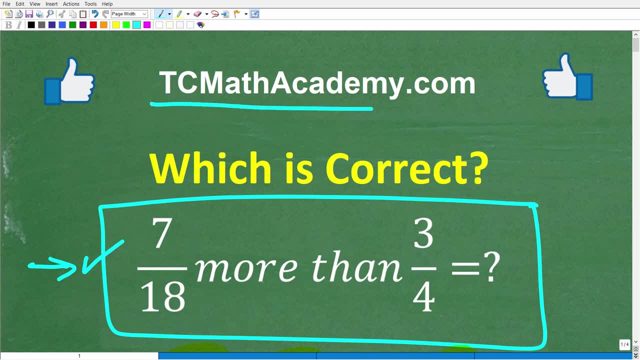 And if you need help learning math, check out my math help program at tcmathacademycom. You can find a link to that in the description below. And if this video helps you out or if you just enjoy this content, make sure to like and subscribe, as that definitely helps me out. 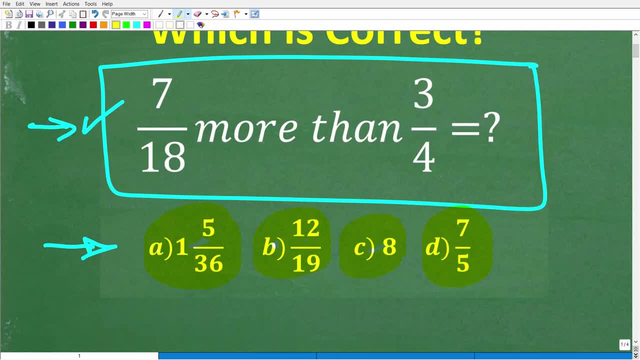 All right. So one more time, we have this problem and we want to know 7, 18ths, more than 3, 4ths, is how much? And we're not going to use our calculator, All right, so let's take a look at the answer. 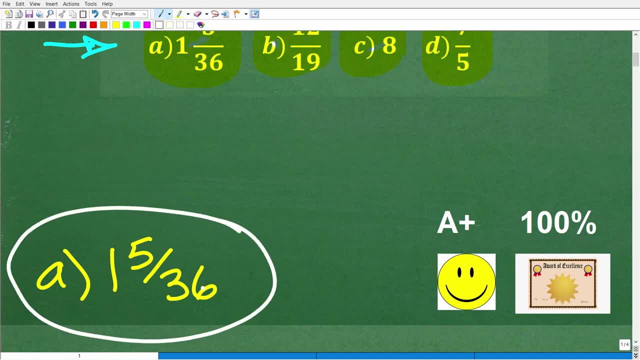 The correct answer is A 1 and 5 over 36, or 5- 36.. So it's a mixed number fraction. Now it's possible. some of you did this right, but you have an improper fraction And an improper fraction. matter of fact, let's have a quick quick. 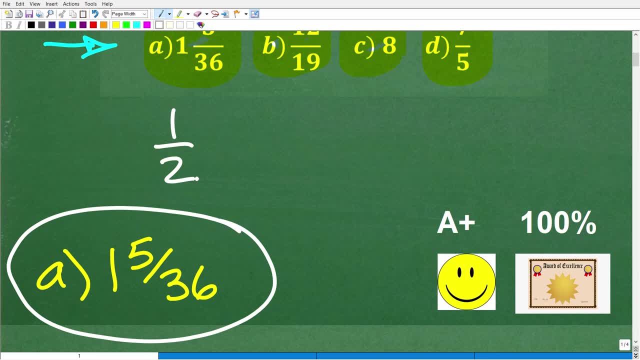 Uh, mini lesson on fractions. So, uh, a fraction has two parts: a numerator and a denominator. The top? uh number is the numerator, The bottom number is a denominator. So when the bottom number is bigger than the uh? uh top number, the numerator. 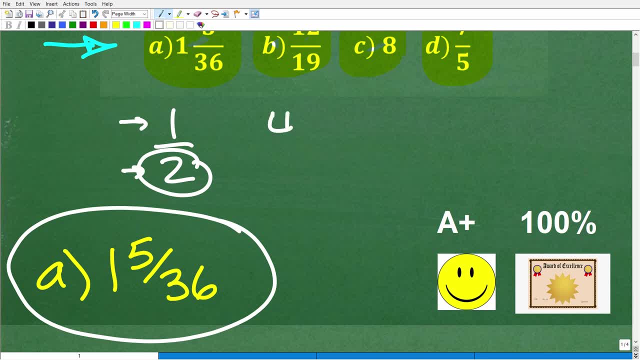 So, like in this example right here, this is a proper fraction. but if you have like 4 over 3, where the numerator is bigger, that's an improper fraction, And these type of fractions can be uh converted to uh, mixed number fractions. 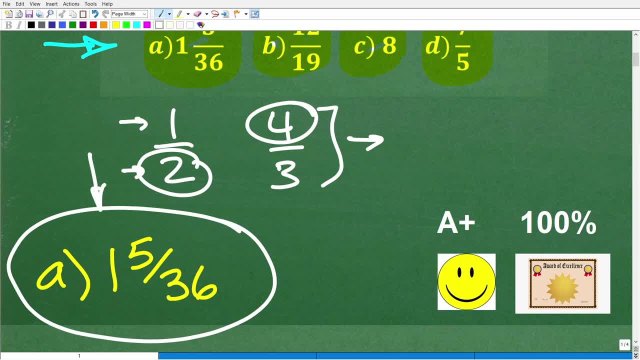 Like this. So we have mixed number fractions, improper fractions, improper fractions. So, uh, double check that. uh, you may have the correct answer as an improper fraction, because we're going to have to do some division here as well. So this is going to be an exciting uh problem for those of you that love arithmetic. 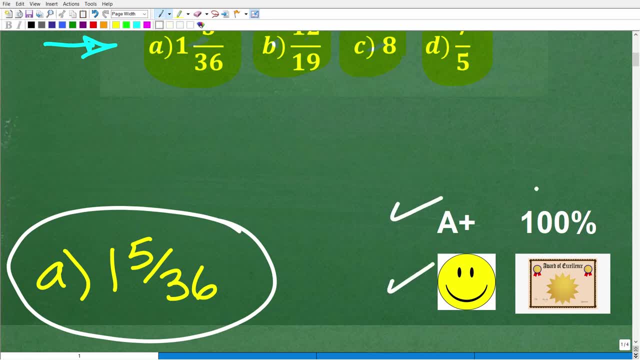 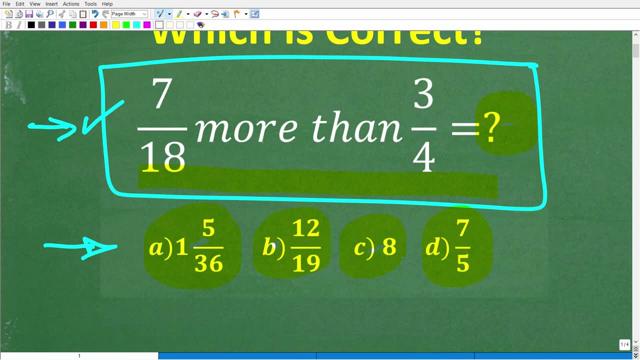 But, uh, anyways, if you got this right, you definitely get a happy face and a plus 100% and a certificate of excellence, because you definitely appear to be a certified professional expert In the area of adding fractions and converting an improper fraction into a mixed number fraction, because this is the answer. 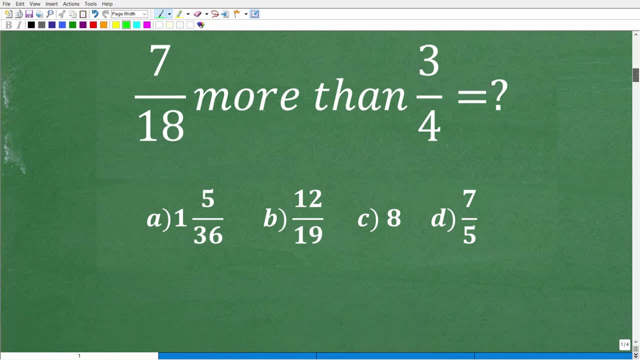 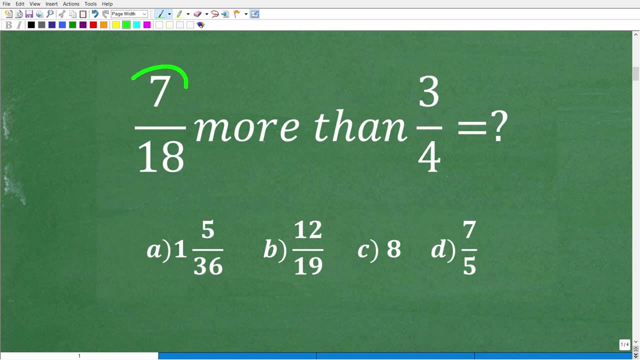 All right, So let's go ahead and get into all this right now. So here is our problem, And the first thing that we need to do is interpret what this thing is saying. So we have 7,, uh, over 18.. 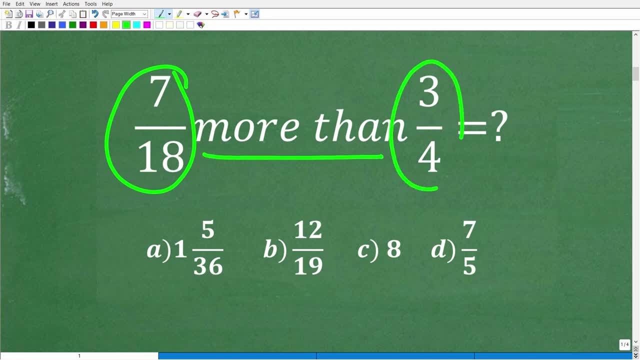 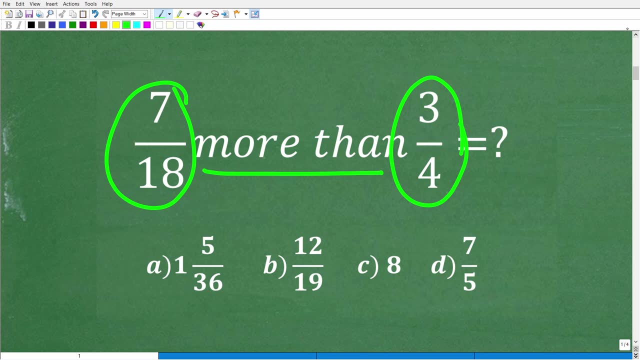 We want 7, 18ths more than 3, 4ths. All right, Now how do we figure What this problem is saying? Well, one thing, that is a fantastic little uh technique that you should use in all math problems when you're confused and you're like: Hey, Mr. 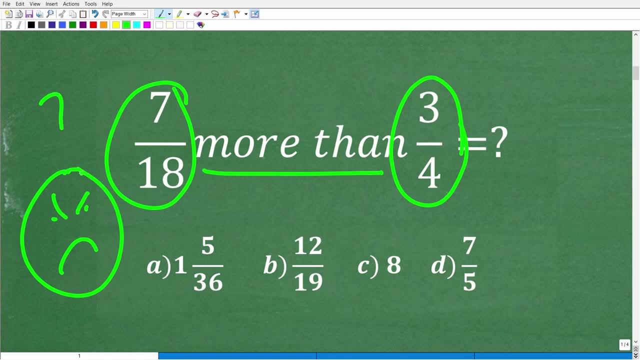 YouTube math man. I'm just generally confused. I have no idea what this problem is even saying. Well, uh, two things you can do. One: we have a multiple choice question. So if you're not even sure and you're taking a math exam and you encounter a question like this and you're like, well you know, I'm just going to take a guess. 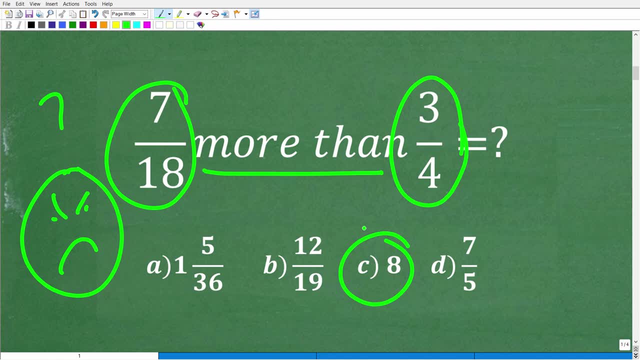 Well, that is not a bad thing. Just take a guess, Unless you're going to get penalized for the wrong answer. So never, ever, leave a math question, uh, blank. Okay, So hopefully you took a guess, but of course this is wrong. 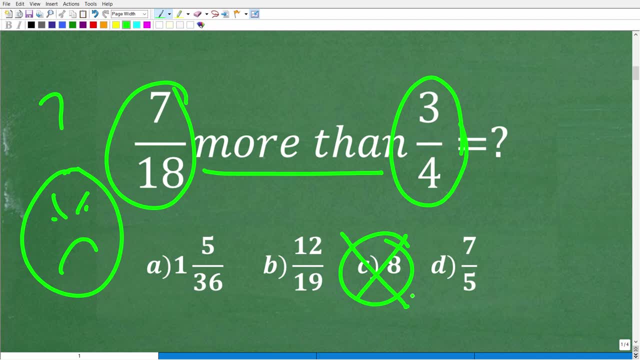 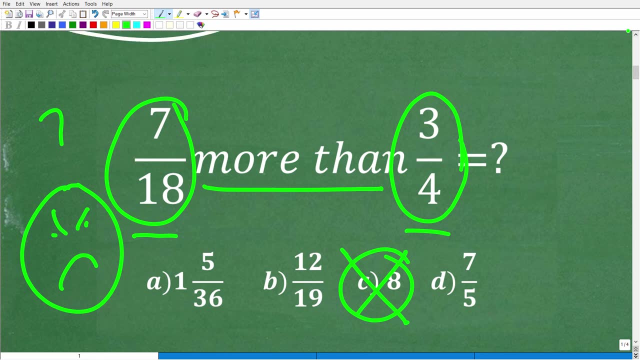 So the only way to know how to do this problem is to understand the math. So this technique that you want to keep in mind is that we have fractions here. So sometimes if you replace- you know- fractions or numbers that are a little bit more complicated with easier numbers and then think about what that means, it's generally, um, you know, um, a path to. 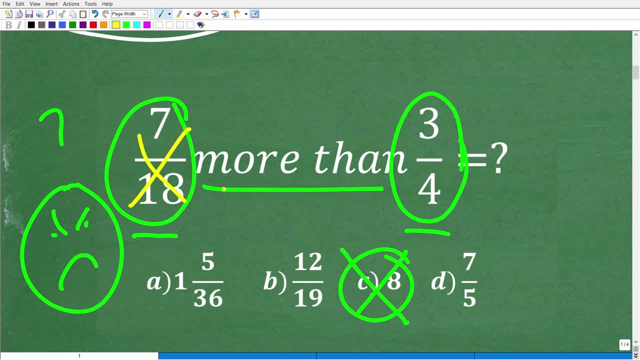 You're figuring out the solution. So, for example, instead of seven over 18, more than three fourths, what about three more than one? or three more than one? What does that mean? Three more than one? Well, if I have one and then I have three more, it looks like we want to add three to one, right? 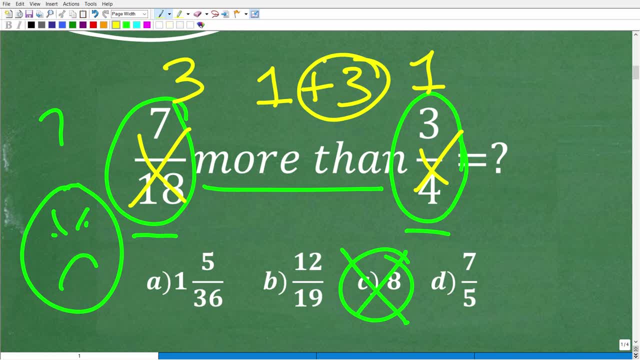 So we're just basically adding these two numbers and because we don't have any negative numbers here, we're not dealing with a subtraction situation. It looks like: uh, all we need to do is simply Add these fractions, And that is exactly what we need to need to do in order to figure this problem out. 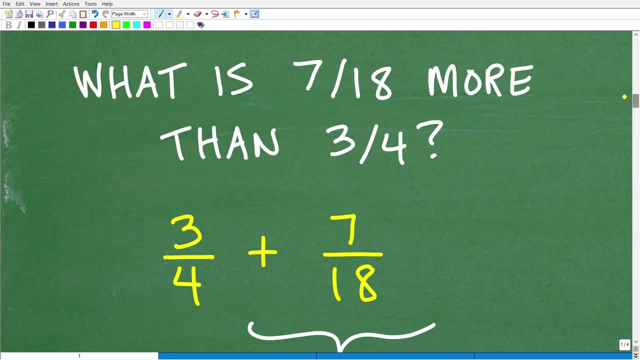 So what is seven, eighteenths, more than three, fourths Again, if you're confused with this type of problem, always just replace these numbers, these fraction numbers, with something easier- And this is a great technique, again with like algebra problems or other problems. 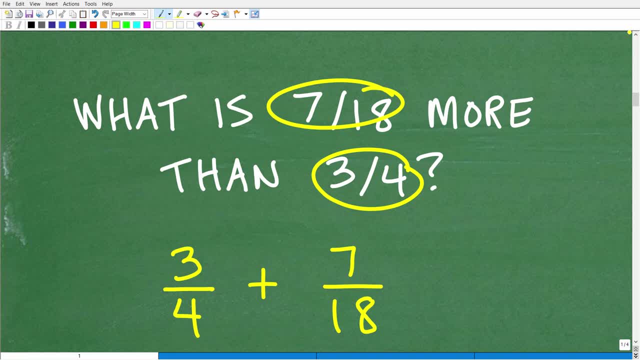 Always try to see if you can construct a simpler version of the problem, to kind of model what's going on. Think about how to solve that, Okay, And then just translate- you know that logic over to your actual problem. right? So like what is three more than one. 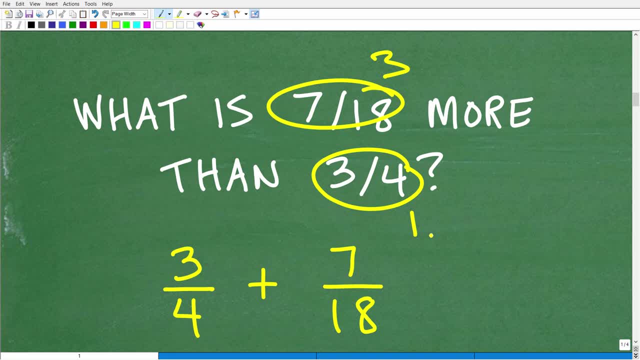 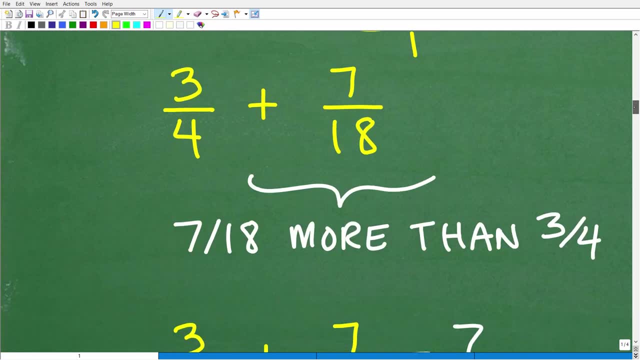 What is three dollars more than one dollar? Well, maybe that's like four dollars, right, Okay? So, basically, here we are adding these two fractions, seven, eighteen plus three fourths, And so now this becomes a fraction addition problem. Okay. 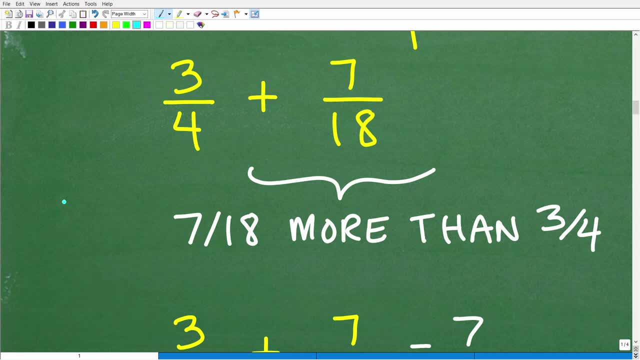 So again, we're not using our calculator here, so we're going to have to figure out what three fourths plus seven, Eighteen, Eighteenths is equal to. So here we have three fourths plus seven- eighteenths, but seven eighteenths more than three fourths is three fourths plus seven over eighteen right. 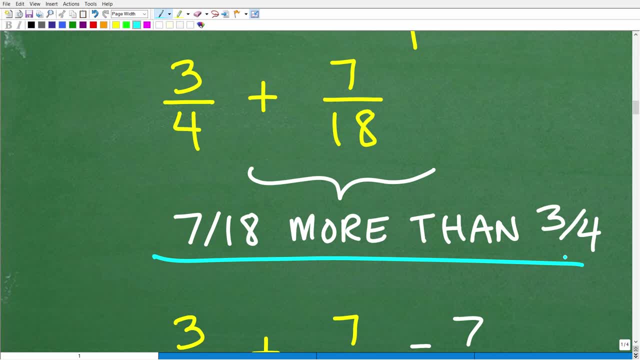 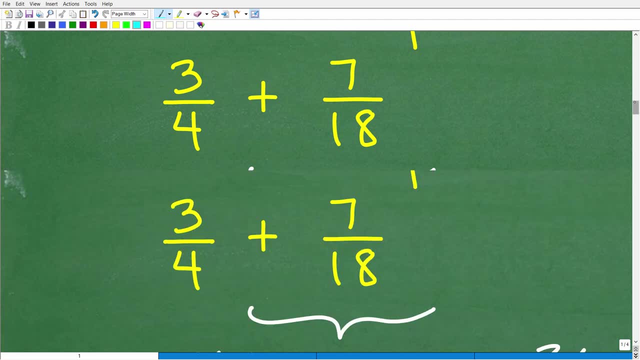 So this is how we have to interpret this phrase. and double, triple, check yourself right. You know write it in different ways. Just you know. have the confidence that you are interpreting these problems. But one thing that you learn in mathematics is how to translate verbal phrases into mathematical statements. 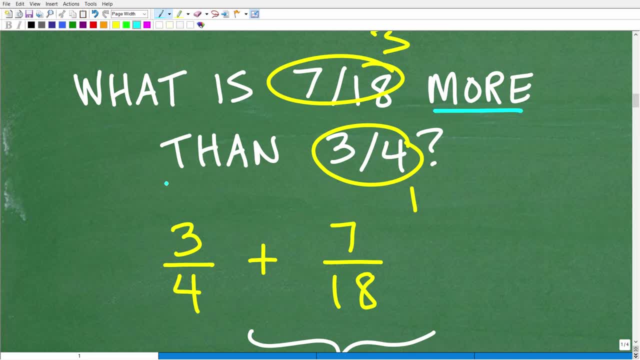 This is really, really critical. So words like more than you know, or the difference of, or the quotient, the product- you know I'm kind of using fancy math terms here, but you need to understand these things. But anyways, I think most people figure this out- that we have to add these fractions. 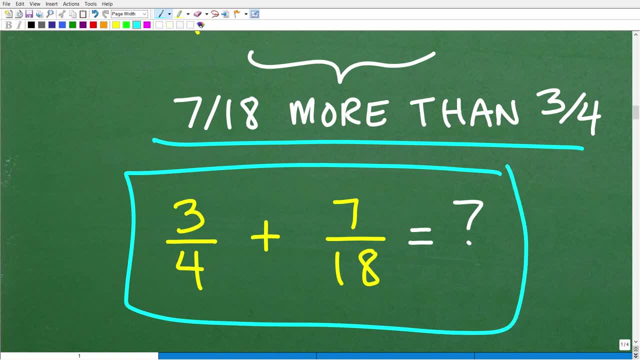 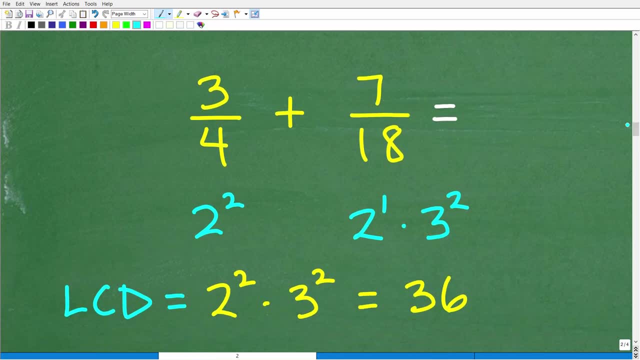 All right. So our problem really is three fourths plus seven over eighteen. And now this is an opportunity for you to show off your fraction skills, Okay, So how do we add fractions? Well, we cannot add fractions, We cannot subtract fractions or subtract fractions unless the denominators are the same. 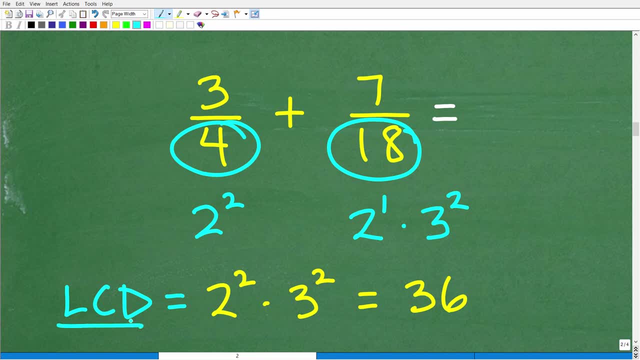 Okay, So you can see, here I'm figuring out the lowest common denominator. So we're going to have to change these fractions, these respective fractions. We have to write them in such a way where they have the same denominator, In other words, four and eighteen, where we have a denominator that has something in common with both four and eighteen. 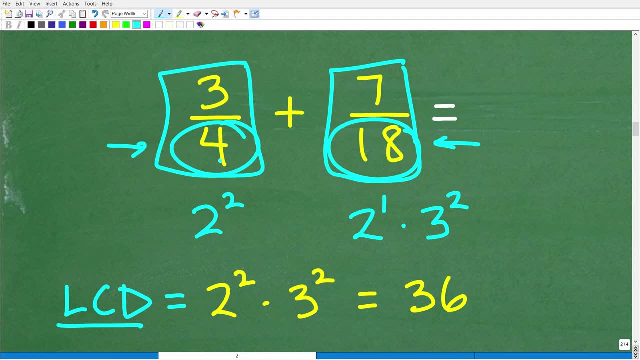 But we want the lowest number that is in common with four and eighteen. Now, technically that's called the lowest common denominator. It's not the lowest common multiple, but really we think of that as the lowest common denominator, right? So this is how we want to approach this problem is, we need to figure out the LCD and then we need to rewrite these fractions such that the respective denominators have the LCD. 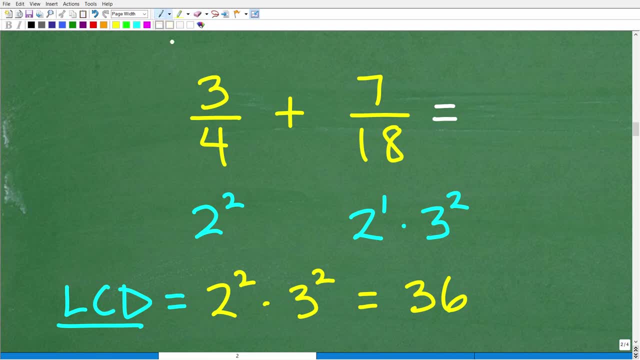 Now you can see I have some work here and that work is how you actually find the lowest common denominator. Now some of you might be saying, oh, I got four, I got eighteen. You know, you might be kind of. 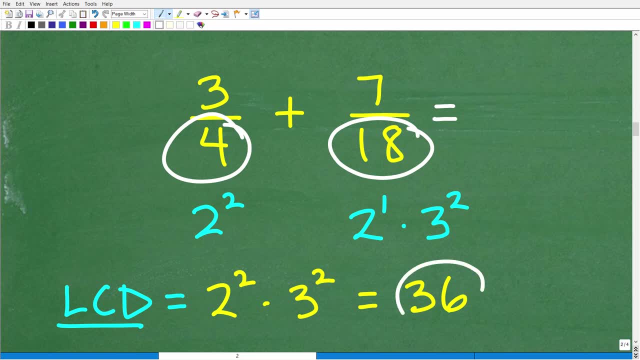 You know doing some number crunching in your brain, Remember, we're not using our calculator, but you could probably have determined that the LCD here is thirty six. So thirty six is the lowest number that both of these numbers can divide into. 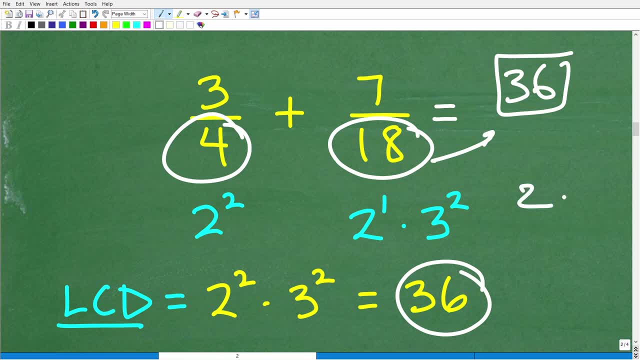 Right. So we can do: thirty six divided by eighteen is two, without a remainder, And then four times nine is thirty six. So thirty six divided by four is nine. So that is another way to kind of think of the LCD, the lowest number that both of these numbers can go into. 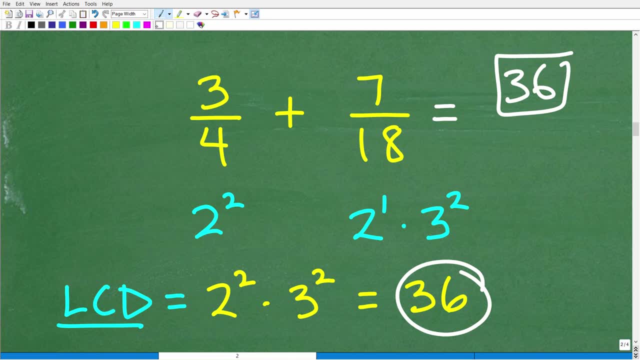 But that's only a way to Think about the number, It's not the procedure on how to find the LCD. Now some of you might be saying, hey, Mr YouTube Math Man, you're rambling too much about the LCD. 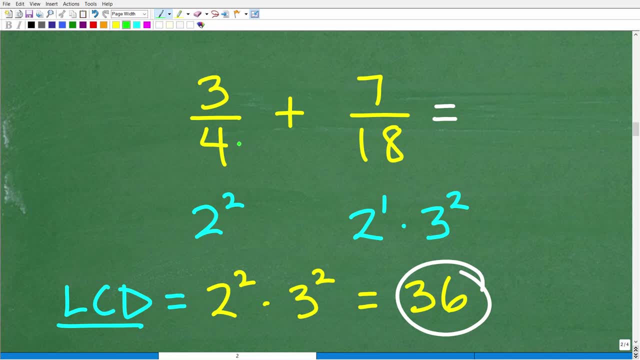 I'm a professional expert. Well, if that's the case, if I gave you like four or eight, three or four or eight plus one, seven over one, eighty two, could you find the LCD? Well, at this point a lot of people would be like, all right, well I'm, I'm unsubscribing. 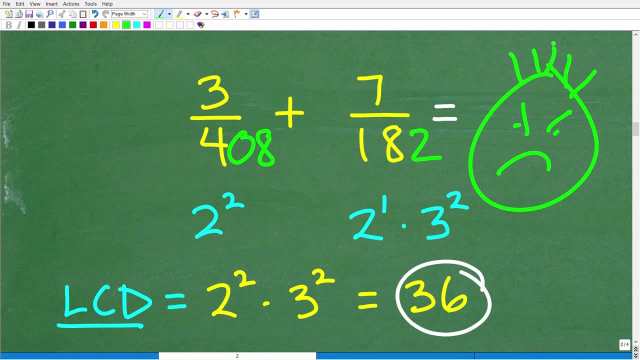 I'm going to leave your video right now, Mr YouTube. Math Man, I don't want to do that problem And I don't blame you. But if you have to do this problem, you've got to understand the procedure. how to find LCD? 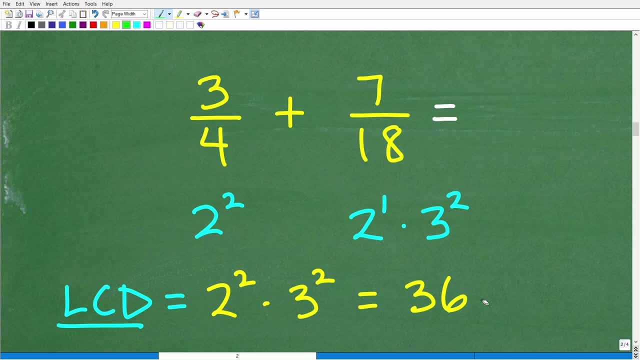 And this is a big, big topic, not only in arithmetic but in algebra. All right, So I'm just going to cover it real fast and then we'll continue on here. But to find the LCD? Now, we already know it's thirty six. 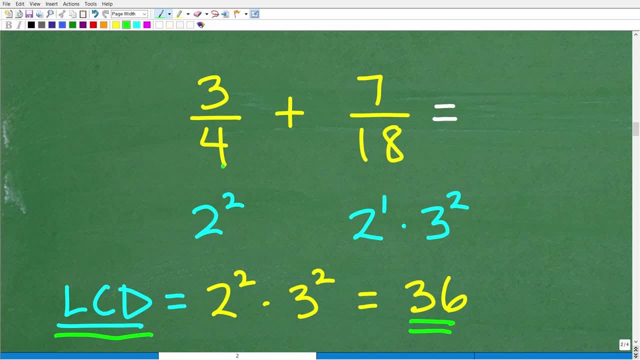 Right, So what he talked about that. But what you want to do as a procedure, OK, is the denominators you want to prime. factor the numbers in the denominators, All right, Each respective denominators. So four is the same thing as two times two. 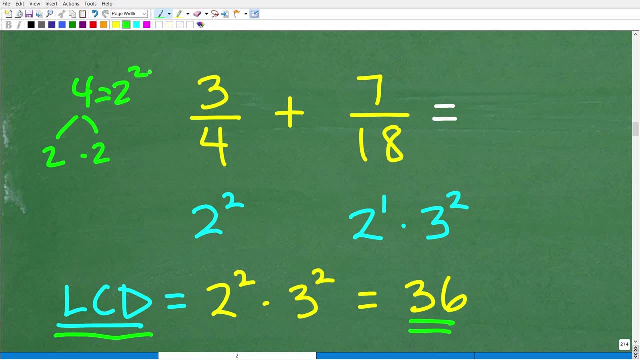 So we can express four as the prime factors as two squared. So we always want to express this in terms of a power, And so four, in terms of its prime factors, is the same thing as two squared. All right, So 18 is what? 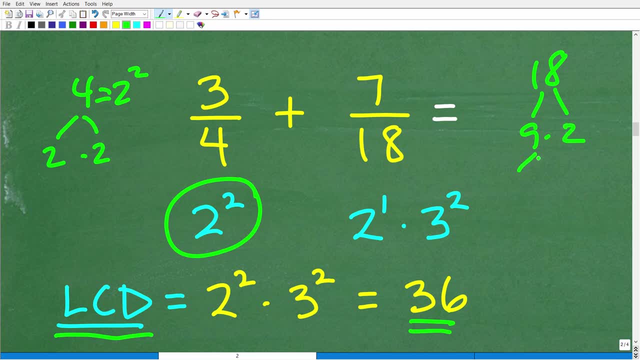 Well, we can be like: all right, that's nine times two, And then nine is three times three, because nine is not a prime factor. So three times three, These numbers are prime. So we can think of 18 as three. 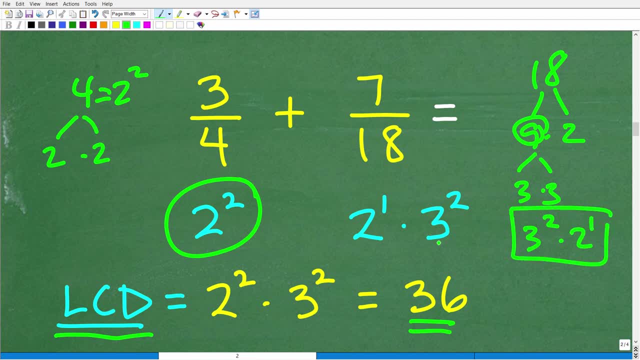 Square times two to the first. Remember, we want all the prime factors of our denominator. So now we have two to the first times three squared, That is 18.. All right, So now we can easily identify the LCD. OK, now the way this works is you're going to take the highest power. 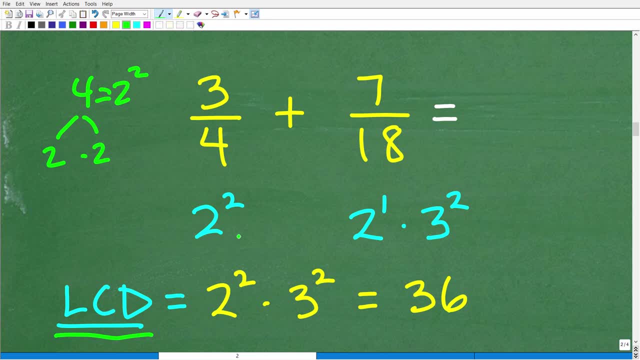 Well, let me kind of back up here. You need to have each of your the numbers of these prime factors represented in the LCD as a product. OK, So in other words, we have a two, we have another two over here, we have a three. 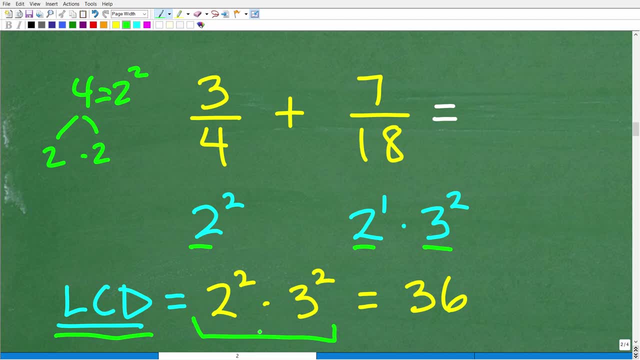 So we're going to need two and three in our LCD. We're going to multiply them together. But some of you might be saying: well, do we multiply two squared, two to the first and three squared? No, no, no. 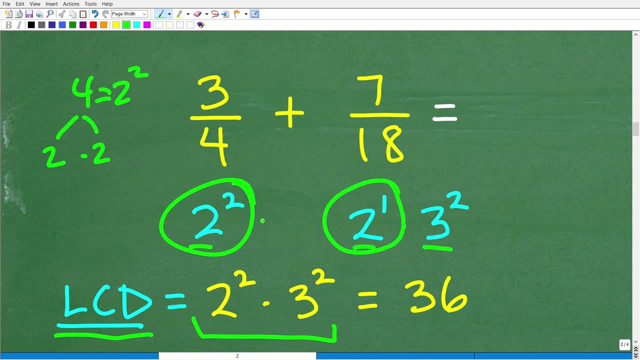 Because we have two, two, two powers of twos here, right? So two squared and two to the first. Which one do we use? Do we use both? Well, no, OK, you only use the highest power. So this is the highest power: two, two squared. 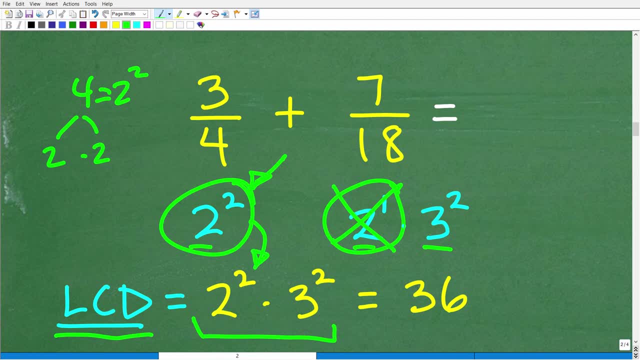 So we use that, We use this in our LCD. So that's going to be two squared, But we need our three squared as well because we need all these prime factors represented. So two squared is what? Well, that's four. Three squared is what, That's nine. 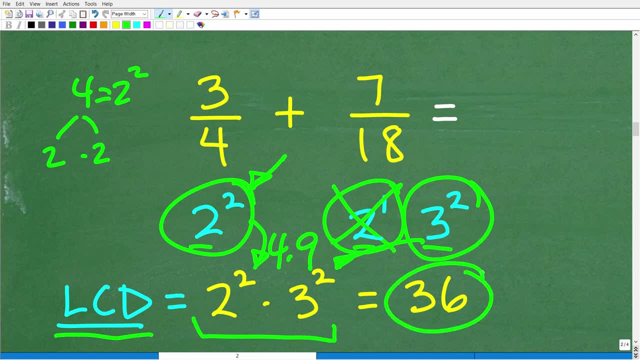 Four times nine is thirty six. This is how you find the LCD. Now again, a lot of people are not going to do that, because they can kind of just determine what the LCD is, because these are basic problems, but as the denominators get more challenging, 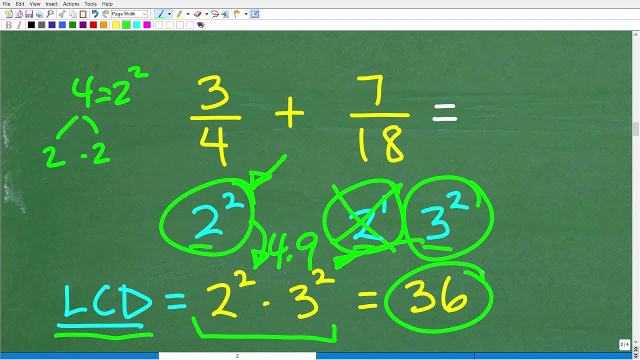 you need to understand this procedure, which means you need to understand prime factoring, and you know, of course, how to build your LCD. Really, really important stuff, But all right. So now that we know the LCD is thirty six, what do we need to do? 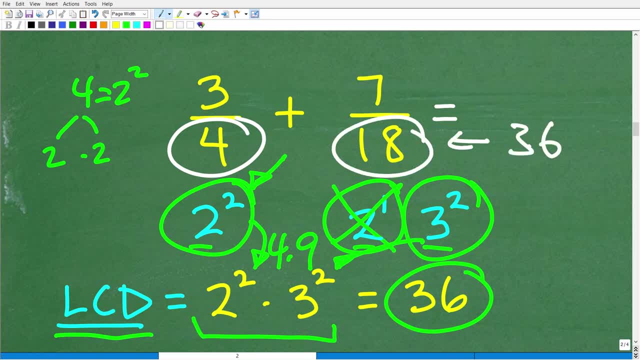 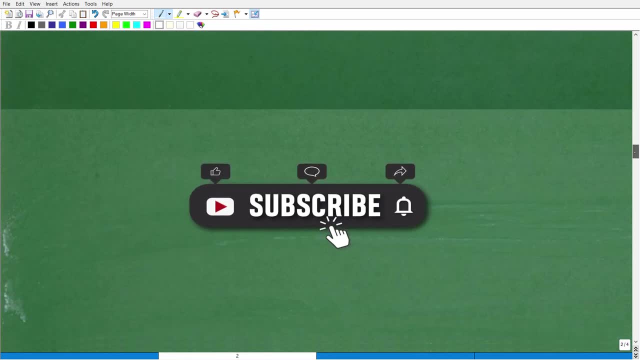 Well, we need to change each of these denominators such that the denominators are thirty six. So let's go ahead and do that right now, OK? so before we get into that, I need you to take a good look at this and say: 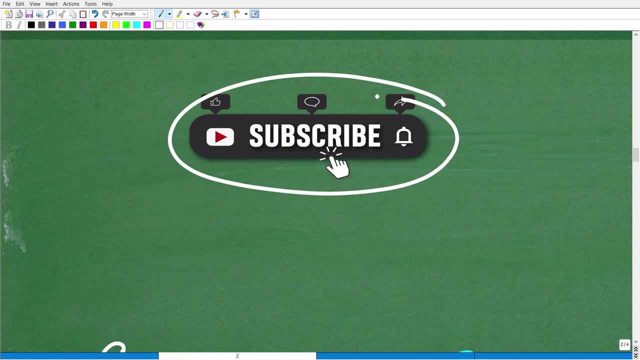 well, I think he's going to ask me to subscribe to his channel, And indeed you would be correct. I definitely need your support. OK, I'm not afraid to ask for help, Right See, I'm not afraid of that work because I have a goal. 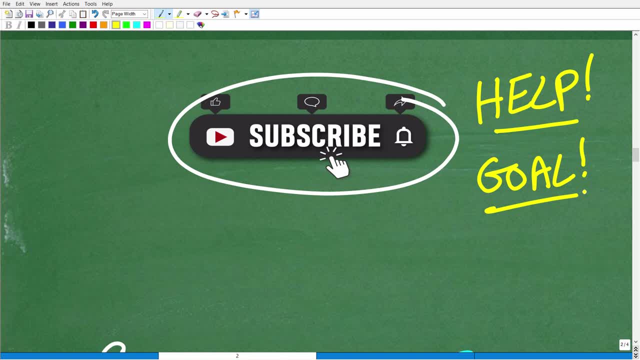 If there's two words that you want to have in your vocabulary, the first is having a goal. now, it could be any kind of goal, but just have a goal in your life, Hopefully. have multiple goals, All right, Maybe you want to get in shape. 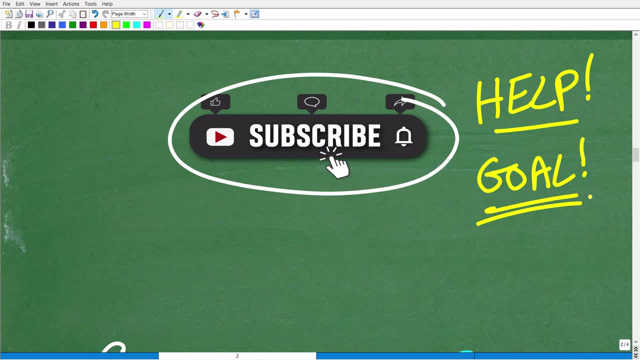 Maybe you want to get better at math. Maybe you want to make a million dollars. Whatever the case is, you need to have some goals, But oftentimes you're going to need some assistance to get to where you you know to achieve your goals. 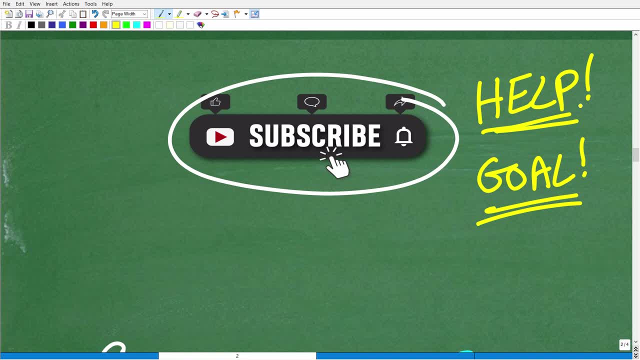 Right For me. my goal is to grow this channel as large as possible because I know I'll be helping more people in math. OK, I'm all about helping people and I actually need your help to be able to help other people, And YouTube really does count how many people subscribe and hit that notification. 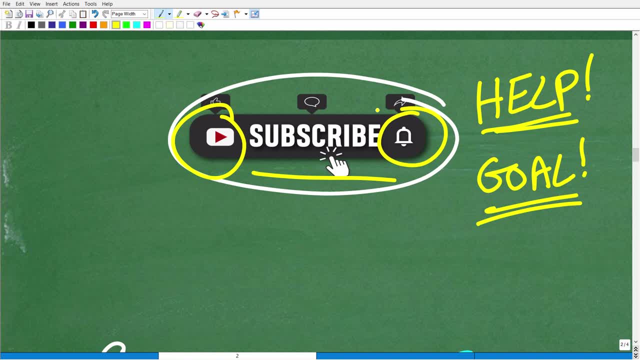 bell. So all these little you know activities on my channel really helps me help other people. OK, and hopefully you're getting something out of this. I'll see you next video, But you know I'm very, very passionate about. 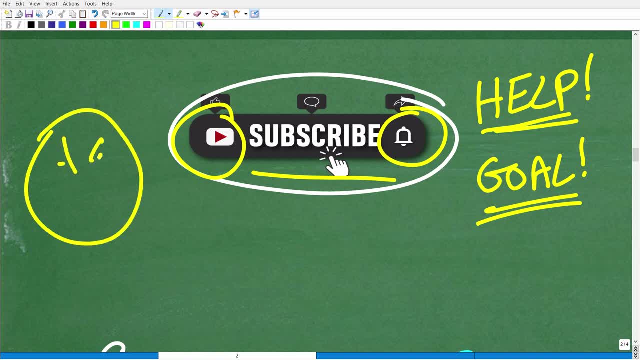 teaching math primarily because math, you know, I mean, I love the subject of mathematics, but I've seen this happen too many times, where people and I have countless- you know- examples of this through the years. Many, many, many. I can't even count how many people I 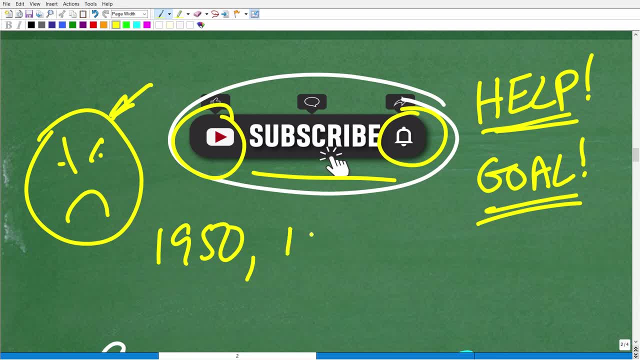 know that had a bad learning experience in the 1950s, 1960s, 1970s were literally some teacher told them: hey, you're bad at math or they failed some math class And no one kind of was there to help encourage them. 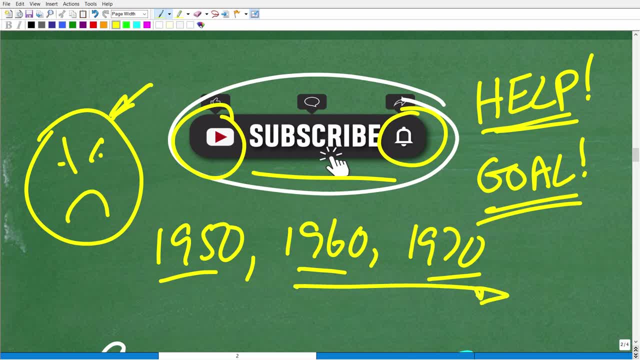 And people struggled for decades thinking they were bad at math And it had a huge impact on their life to the degree where you know. maybe they they went off in a different direction, Maybe they wanted to be an engineer and they didn't. 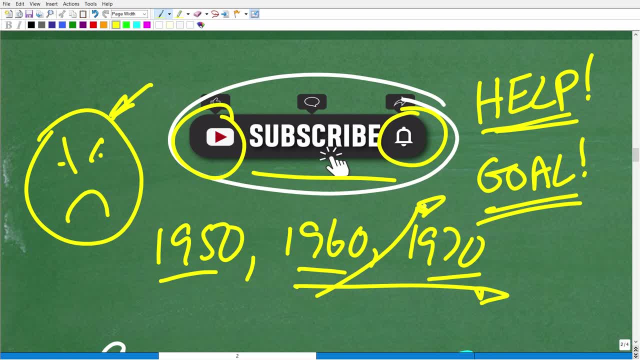 And I'm like boy if it was just one. you know, teacher or something happened can have a huge impact on the trajectory of someone's life. So I'm very passionate about encouraging people that don't give up on math if that's what they want to do. 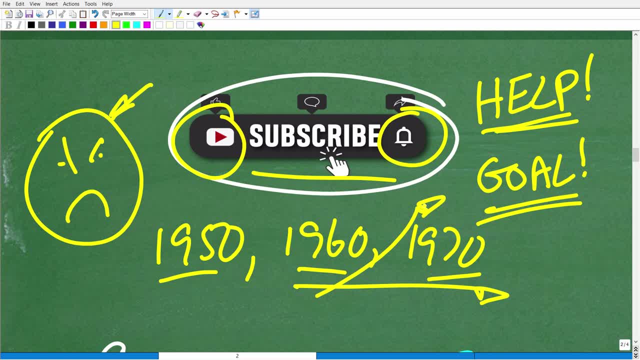 If you want to learn math, you can be successful. So don't let anyone tell you- especially a math teacher or anyone say that you can't be successful in math. I'm here to tell you that you absolutely can, But it takes work time. 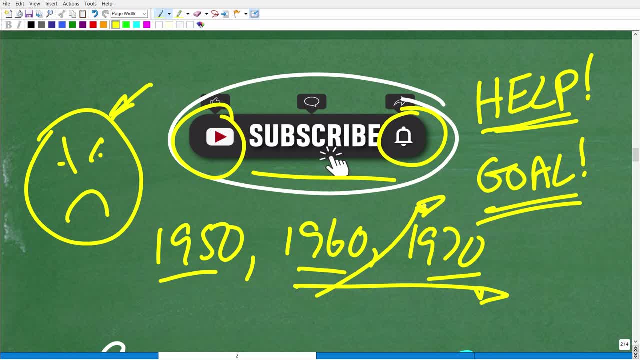 And, most importantly, it takes great clear, comprehensive math instruction that you can understand. So if you're interested in learning more mathematics, check out my full main math courses. You can find links to those in the description of this video. Matter of fact, the things that we're talking about here is like basic math. 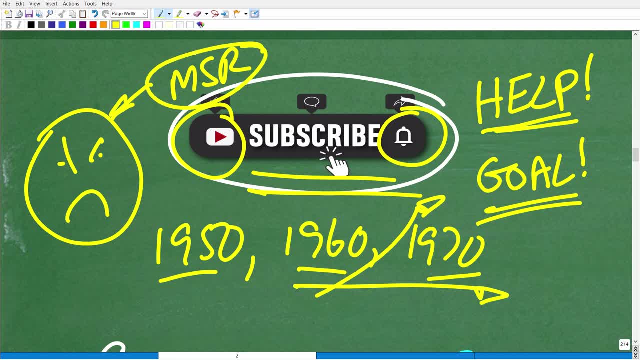 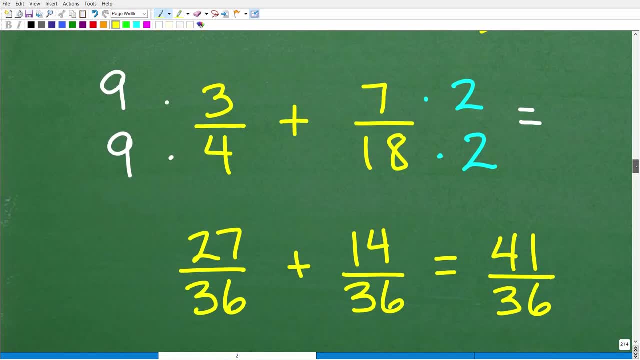 So, for those of you that want to relearn math, I want to check out my math foundations or math skills rebuild. Of course, I cover all this LCD fraction business, But let's get back to this problem here, All right. So now that we know that our lowest 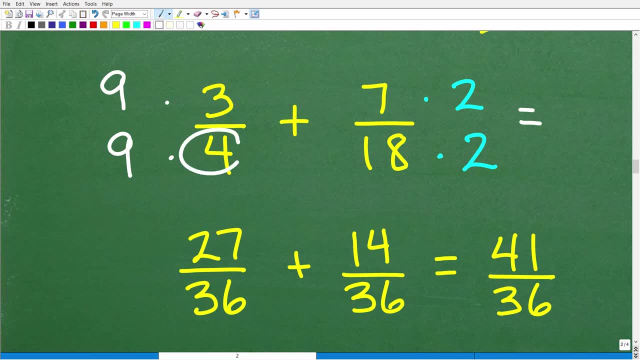 common denominator is thirty six, we need to change each denominator such that it's thirty six, All right. So how do we change a four to thirty six? Easy, We need to multiply it by nine. So that means we need to multiply the numerator by nine as well. 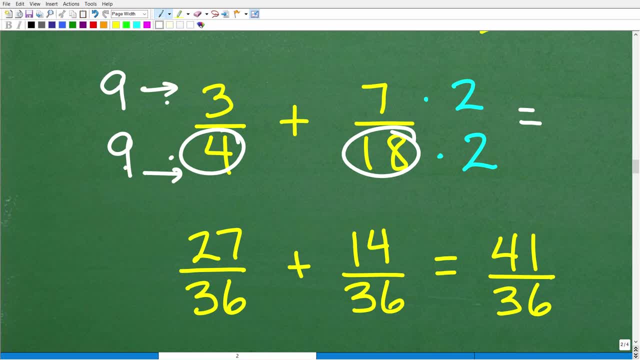 Remember, when we're rewriting equivalent fractions, whatever we need, whatever adjustments we need to make, has to be the same for both the numerator and denominator. So nine times four is thirty six and nine times three is twenty seven. So we have twenty seven over thirty six. 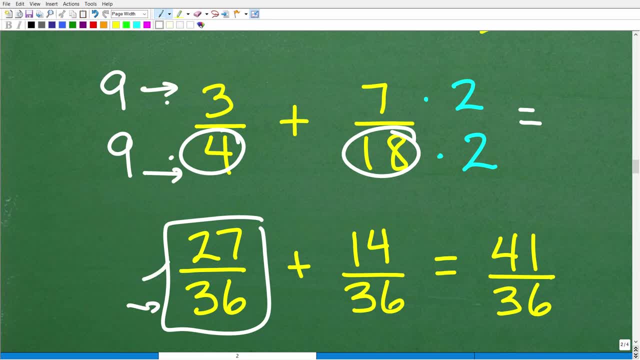 If you saw this fraction walking down the street, you'd be like, hey, I can simplify you, I can reduce you down to three fourths. Right, So they are the same fractions, But this fraction has thirty six as its denominator. 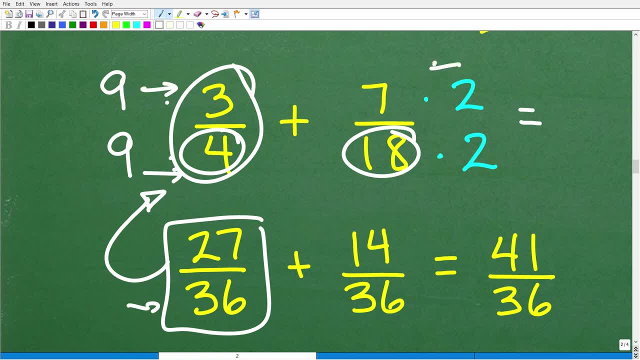 OK, so how do we change an eighteen to a thirty six? going to multiply by two, So we're going to multiply the numerator by two, So we're going to end up with fourteen over thirty six. And now we can actually add these fractions because the denominators are the same. 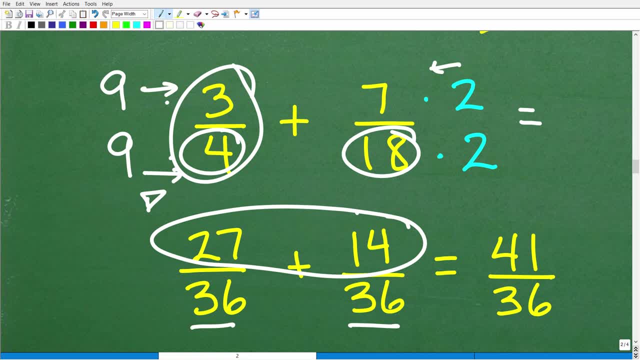 So what you do here is add the respective numerator. So twenty seven plus fourteen is forty one over thirty six. Now, if some of you got to this point, that is fantastic Matter of fact. I would give you a happy face. But here is a problem. 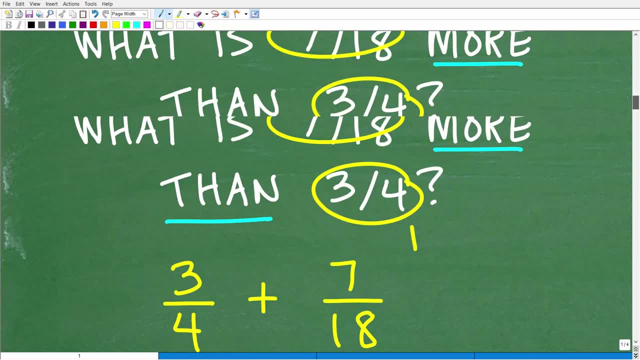 OK, this forty one over thirty six was not a choice. Let's go back over here to the question on our exam, And this can happen. You're like? all right, I'm looking for my answer here. I don't see it. 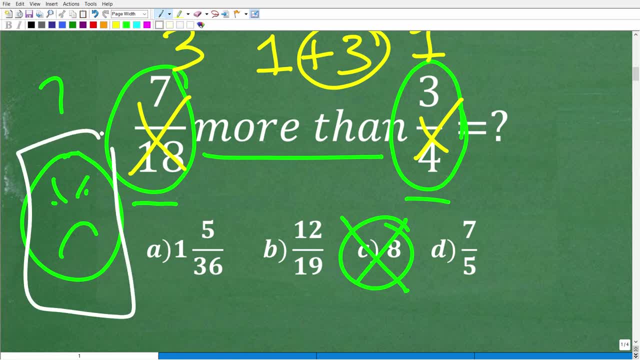 I don't see it. What's going on? You know? did I do this wrong? No, no, no, no. What you have to do is look at the answer, But like, well, maybe this is the correct answer. 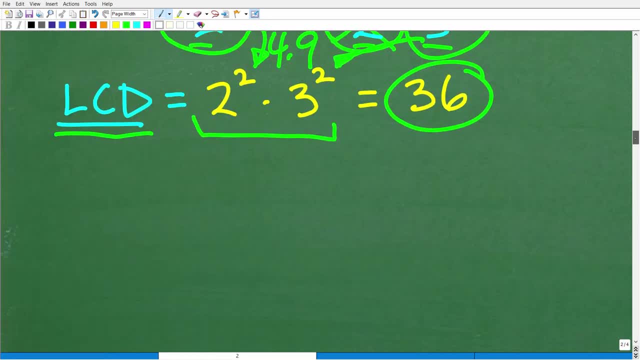 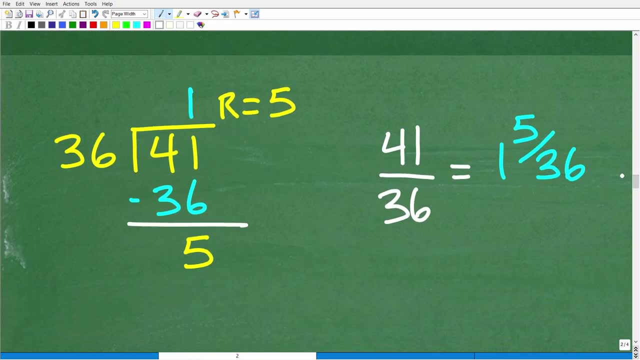 It's just in a different form, And that happens all the time in math. All right, So we're going to have to take the next step here. So forty one over thirty six is correct, But that is an improper fraction, Right? 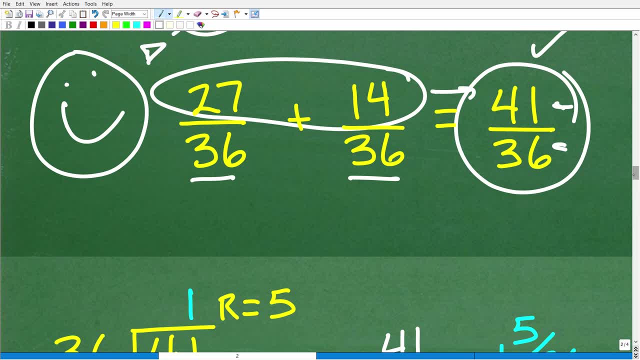 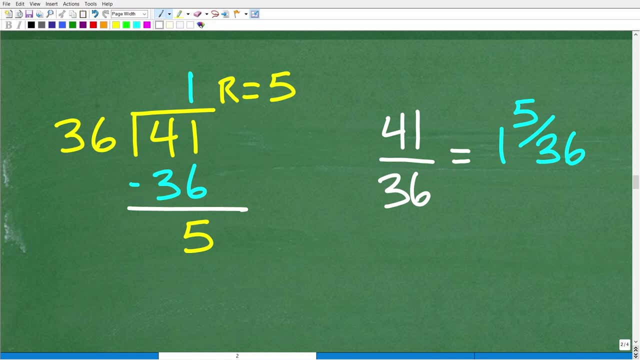 So in other words, the numerator is bigger than a denominator. So we could change this to a mixed number fraction. And how do we do that? Well, we just do some old school basic division paper and pencil kind of stuff. So you're going to take forty one divided by thirty six. 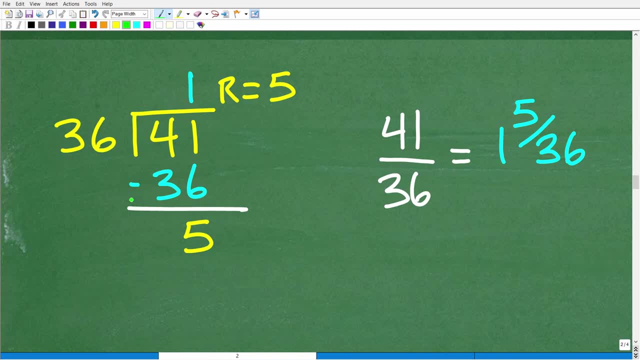 So thirty six goes into forty one one time. So one times thirty six is thirty six We're going to subtract and thirty six, We're going to subtract thirty six. forty one, We get five. thirty six can't go into five, So we have a remainder of five. 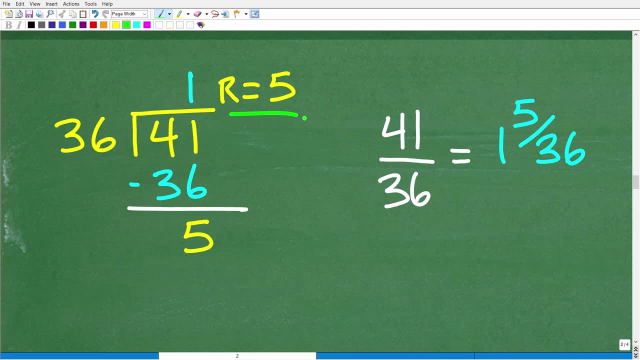 So the forty one divided by thirty six is one, remainder five, But this is not the way we write it. OK, so forty one divided by thirty six- again, This is equal to the fraction. Forty one over thirty six is one. Now the remainder is going to be. what we're going to do is going to write one.